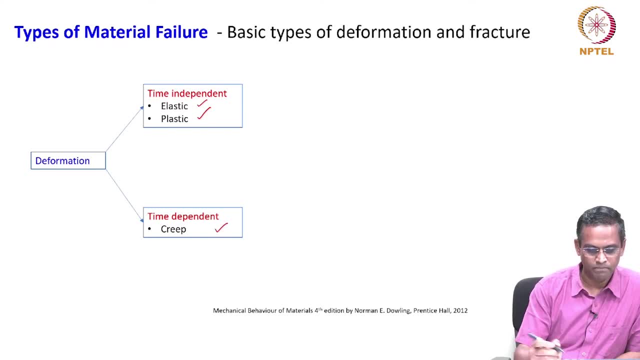 And time dependent is crepe. So materials undergo elastic deformation. You know, most of the material undergo elastic deformation. Okay, And and materials also undergo plastic deformation. this is which what. this is what we want to avoid in an engineering component or structure. we want to avoid plastic deformation. 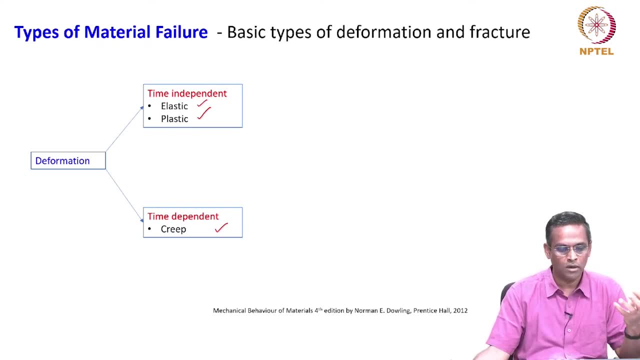 But we should know what, under what circumstances this failure occurs. that is the essential of this subject. So these two deformations, whether it is elastic or plastic, is a time independent. it is not depending upon time. So, on the other hand, the deformation can be time dependent. So 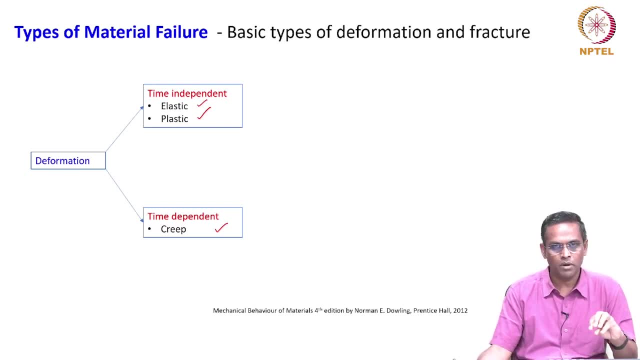 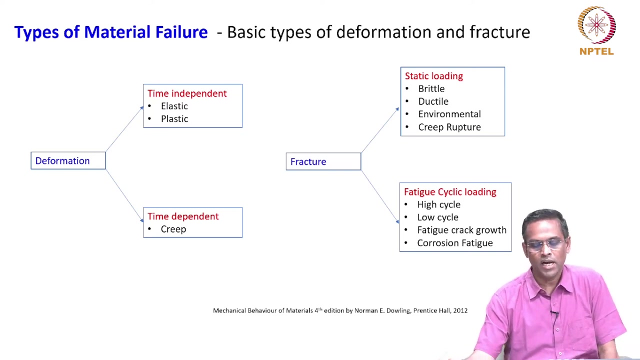 the one of the primary engineering property or failure is creep. it is a time dependent deformation. We will slowly look at it. So, on the other hand, if you take the fracture, you can look at it at in two broad categories: whether fracture occurs under static loading. 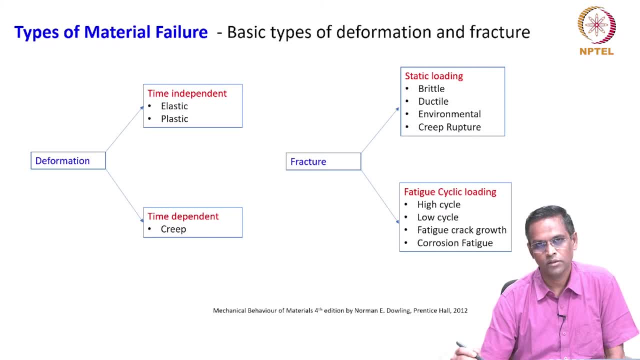 or fracture occurs under cyclic loading. So there are two possibilities. So under static loading the fracture or failure can be brittle in nature- brittle in nature or ductile in nature, or it could be environmental or creep-lupture. So some of these terms are becoming more technical now. 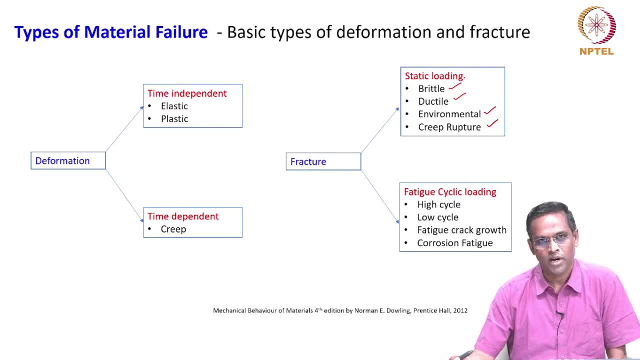 So we should know what is brittle fracture and what is ductile fracture. Brittle fracture is something what we have just seen in the spectacular failures photos, like you know, the ship becomingETH in two pieces. you know, without any warning, you know two pieces brittle fracture. 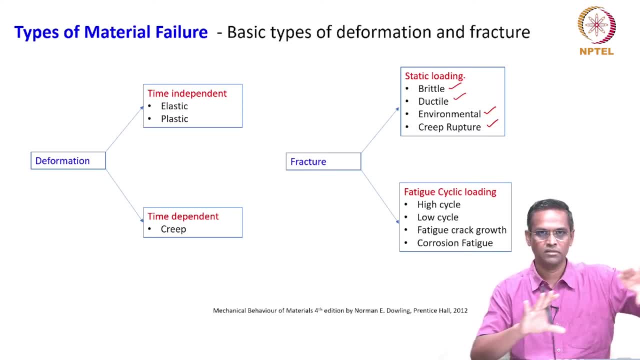 Ductile fracture, the pipe you have seen, with the large deformation you know. and then environmental is, you know, corrosion, you know it could be oxidation corrosion, you know, hot corrosion, and so on. Creep rupture is, like you know, time dependent, as if you keep on, you know. 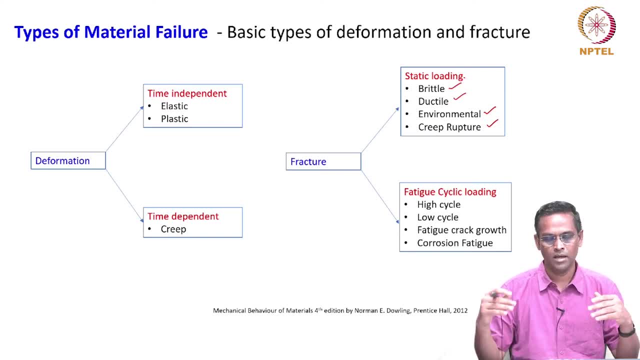 if the component or in structures are subjected to a deformation at high temperature over a period of time, then this is this type of failure coming to each other and coming to cyclic loading. it is called fatigue. Fatigue is cyclic loading. it can be high cycle, low cycle fatigue crack growth. 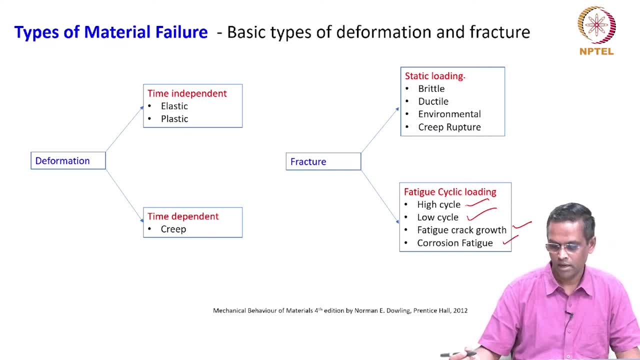 corrosion fatigue? Yeah, we will. we will get into this details of each one of aspect. but high cycle generally, you know it is a stress control fatigue normally. For example, you know the components which undergo stresses within, you know, elastic region for a very long time. right, that is stress controlled, right? 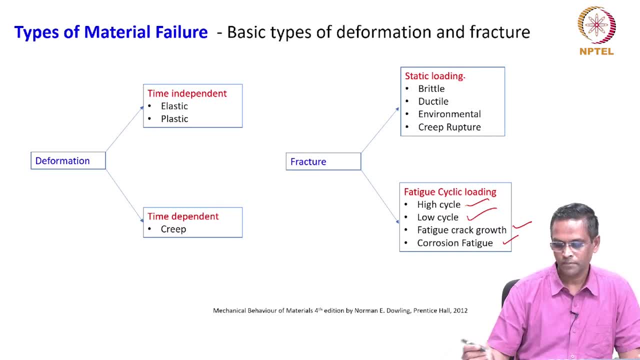 So low cycle means the very word you know says that you know the material will sustain only very low number of cycles. that means you know. that means the stresses are very high. we will be. this component is undergoing cyclic loading- much more plastic deformation or a strain control strain. lot of plastic strain is cycled. we will see it all those in details. So the 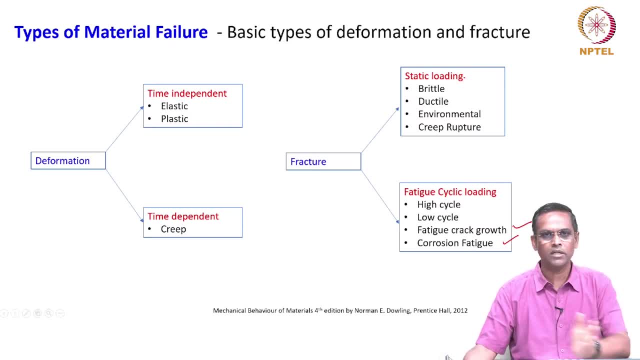 high cycle means that means the components will, will sustain quite a bit of, or quite a number of cycles, very high cycles, right, so that because the material itself is within the elastic region right before yield point, okay, So we will see that when it comes to that point, Fatigue crack growth. so we just- I just mentioned a couple of times before about this- 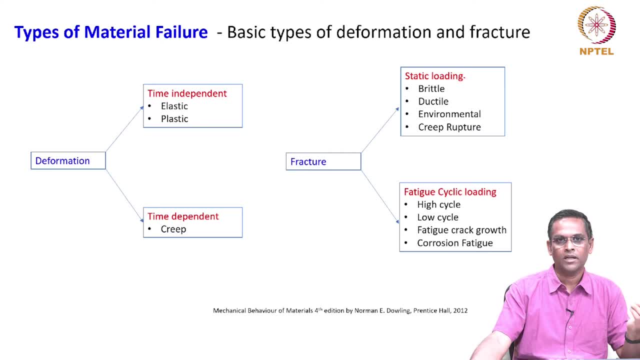 you know flaws and critical flaws and so on. right, So a flaw will grow. when it is there in the component or any structures or vehicles which is under use, the flaw will grow, okay, But how much? you know what is the speed of the growth? okay, and at what condition it becomes. 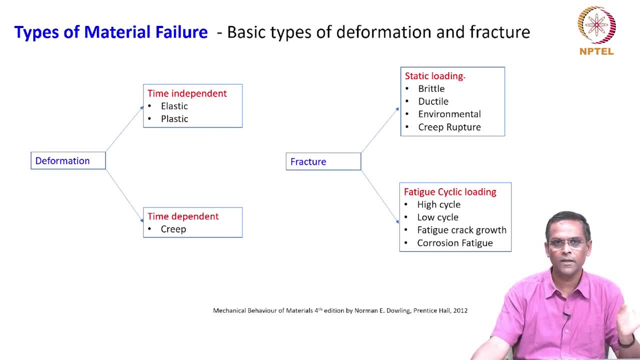 critical or it attains a critical size. these are all the important idea, right, very, very important right. The fracture mechanics: you know subject greatly deals with this and helps engineers to predict some of the life of these structures, right, very important right. Similarly, the corrosion fatigue. so corrosion is 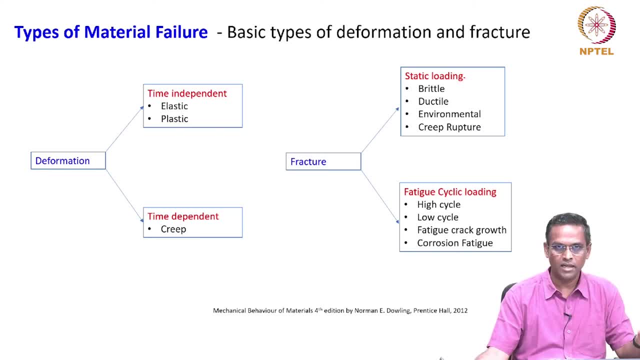 also, it can be static as well as cyclic, so that is why it came under environmental heading. in the static loading- But in cyclic loading as well- the corrosion fatigue takes place. so this is also having primary primary, I mean it is also finding primary concern in most of the 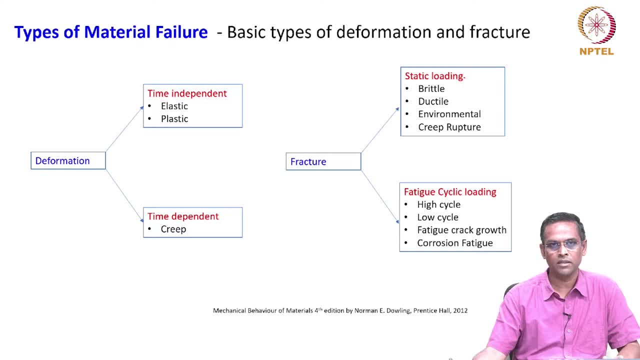 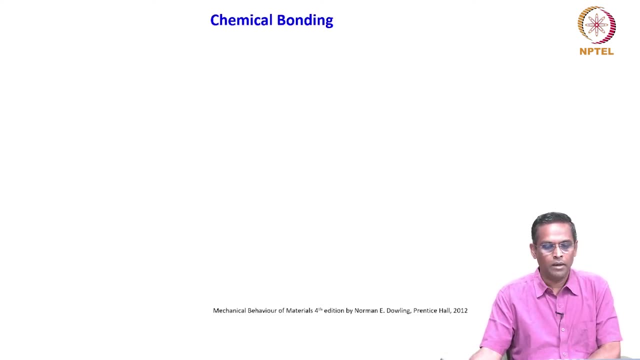 power plants kind of environment where you have materials undergo so stresses are loading current flights and devices like that. So for all those buildings that are such a impact- clase systems, low� Duels- we are still using the pains of the Emotion, Yeah. Very good. I mean, Motor evaluations may not be good. I mean the things will eventually come true, but we still will be working on the problems later on, I think, and if we get into some moments where maybe we could not be, object doesn't be宣言. 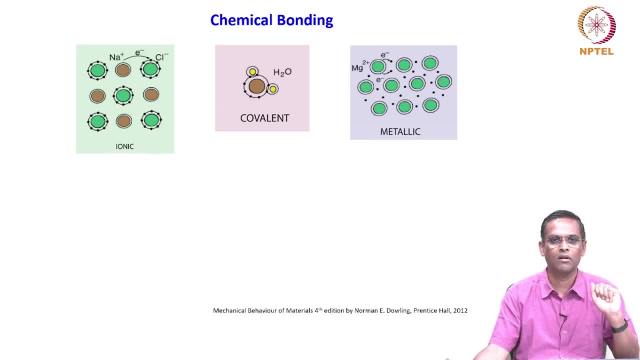 stress is our loading and severe environments right, so that is also very important. okay, Before we get into the real syllabus or subjects, as I mentioned, we will spend lot of time on fundamentals. We will start with scratch, chemical bonding right all of you are familiar with, so that it is always good to start. 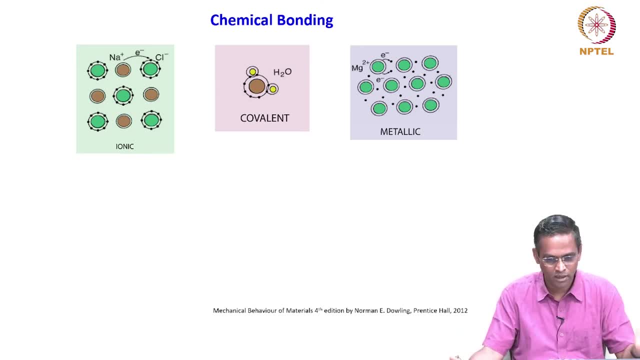 with something, if you are familiar, right, and then we connect: how, how, why do you want to review this? what is the connection of chemical bonding with mechanical behavior? that is exactly i want all of you to understand. that is a strong connection. okay, so let us now review. what is the chemical? 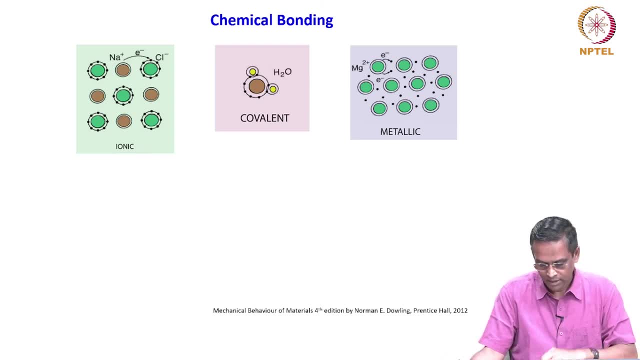 bonding. see, all of us know that there are primary chemical bonds and secondary chemical bonds. the what we are seeing here is ionic sodium and chloride ions, which exhibits ionic bonding. the second one is a water molecule which exhibits a covalent bonding and it is a metallic. it is a magnesium alloy, magnesium metal exhibiting a metallic bond. okay, 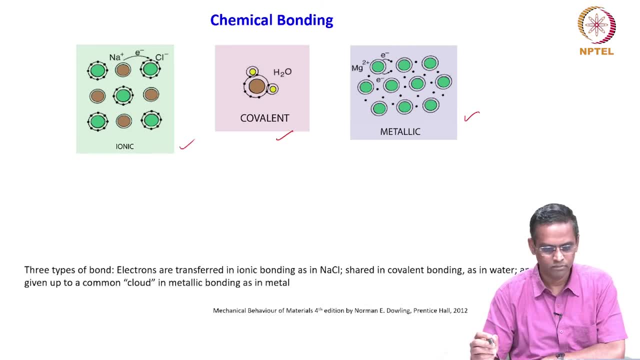 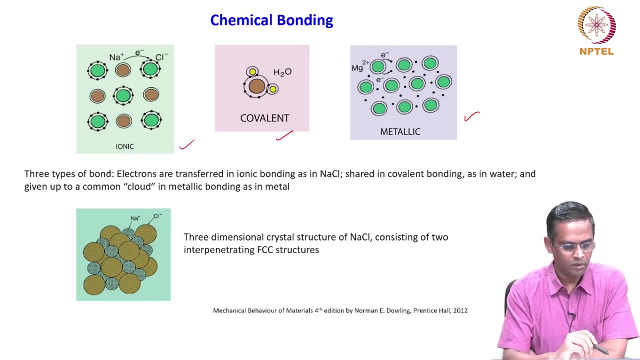 so we will slowly describe this bonding. what is ionic bond? ionic bond is, you know, electrons are transferred in ionic bonding as in in it. that means the- you have this, you know- sodium ion and chlorine ion. so electrons are transferred from sodium to chlorine. okay, so it is completely transferred. 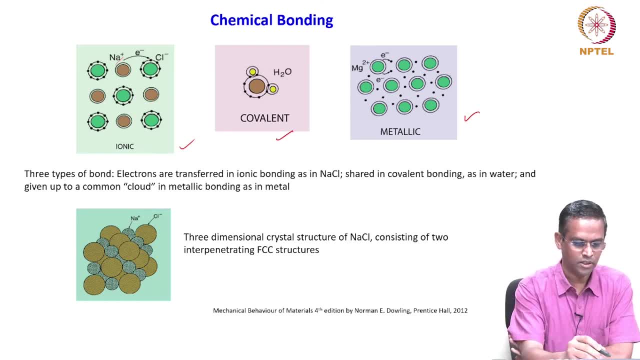 then they stay as ions. that is why it is called ionic bonding. yeah, so when it comes to water, the the bond between the hydrogen and the chlorine is the electrons are shared. okay, the electrons are shared in the covalent bonding, as in water, but the water has got some more typical. 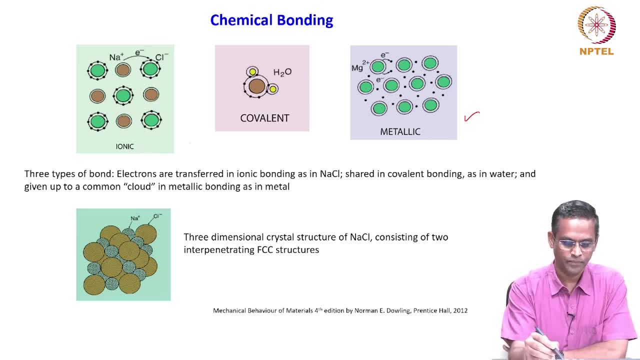 interesting properties. what you see here is see this bond is covalent bond most of the time. it is covalent bond seen like a. but what is also very all of you would have studied this is also will exhibit a dipole moment. right? so you have this hydrogen atom and the, this portion of oxygen. oh sorry, 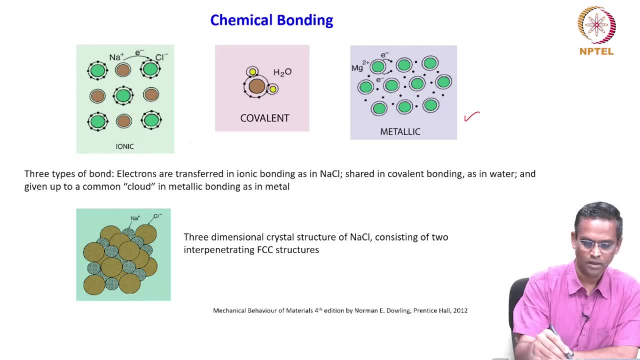 yeah, this portion of oxygen will have negatively charged because of this electron- excess electron here- and asked that because the oxygen is charged in knight tried to fill up around this oxygen collector that actually have done a discharge ボ, do you know fusion on top of this, sorry, you know silicon pot. got cut deeply, because so, if and when we talk about in person observation, oxigen is etapation for mugging sulfate antifungusaters is a position of oxygen absorption, and so you have to be careful when you have, say ó of oxygen frog and latitude is increasing ψ volume. 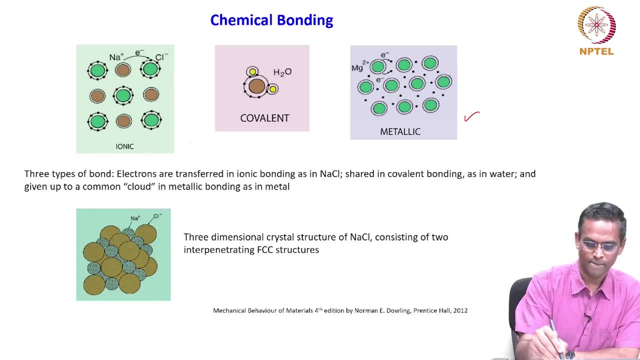 then you do not get witness not found that other anthropomorphic annually and you cannot get a definition also of the bluetooth was a differs and this side it is positive and this side is negative, So it will be a dipole moment, a permanent dipole moment. So water is also called a polar solvent. 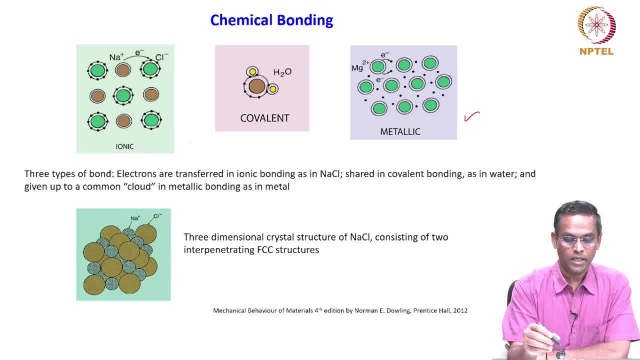 so all of you know. So here we are showing the hydrogen, I mean, here we are taking water as an example. but any molecule which exhibit this kind of a dipole also will form a bond. that is secondary bond. anyway, we will talk, we will discuss that in the next one. 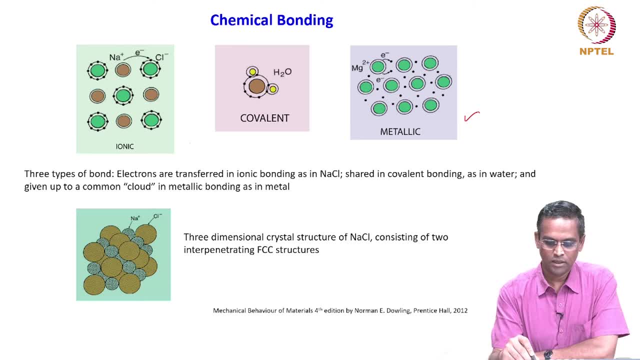 So the covalent bond is shared, electrons are shared between them. And what is metallic bond? Metallic bond is given up to common cloud, So it is a very general description. So what it means is: your ions are there, positive ions or the metal ions are there, they are embedded in the sea of 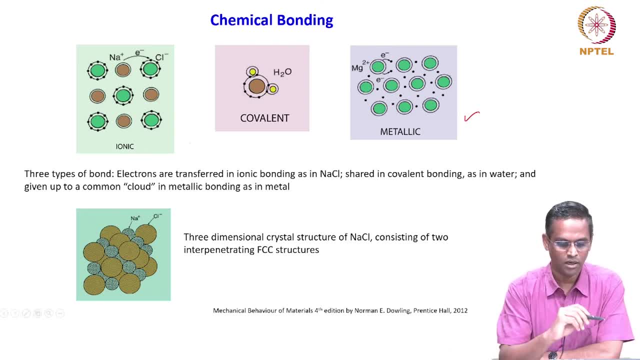 electrons. So that is called, described here as a cloud. So this and all you all know it. but our idea here is: each one of this bond we will connect to its strength and mechanical behavior. that is the idea. So here is the three dimensional crystal structure of sodium chloride. 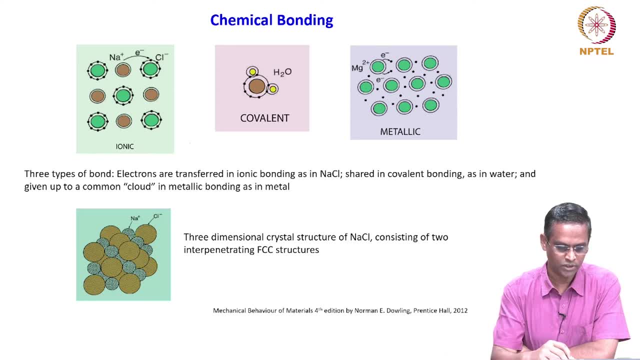 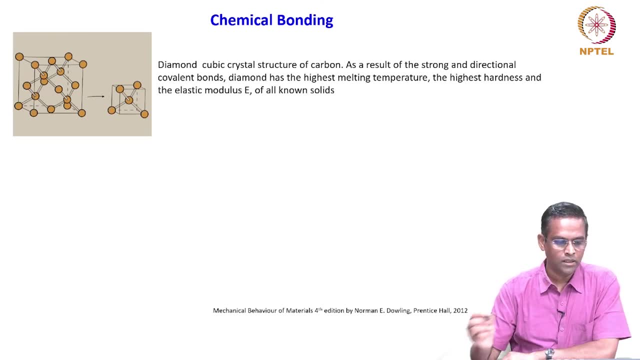 consisting of two interpernet rating FCC structure: vain, solid. So what you are seeing here is another very popular crystal structure or material, I would say diamond, which has got a diamond cubic crystal structure of carbon. It is an allotrope of carbon. 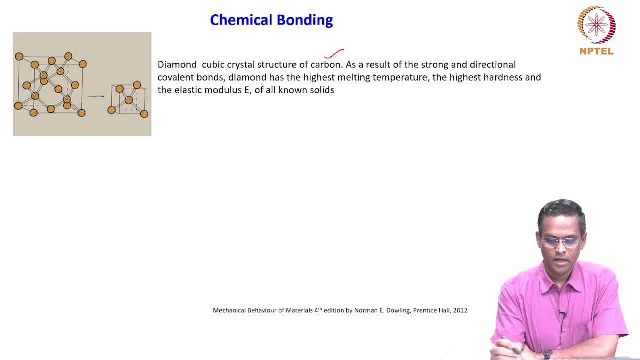 all of you know this- 事項 ל� déb�- as a result of a strong and a directional covalent bond. So this is one interesting aspect of covalent bond which is relevant to any mechanical behavior. Covalent bonds are. 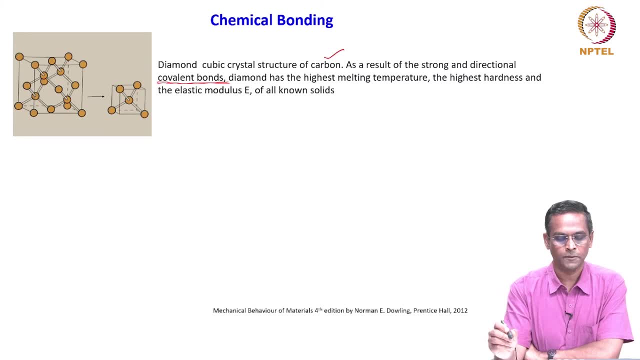 directional in nature and they are very strong and that is why diamond has got the highest melting point or melting temperature, and it is also having highest hardness and elastic modulus of all known solids. So it gives some idea if you have a covalent bond in all directions. 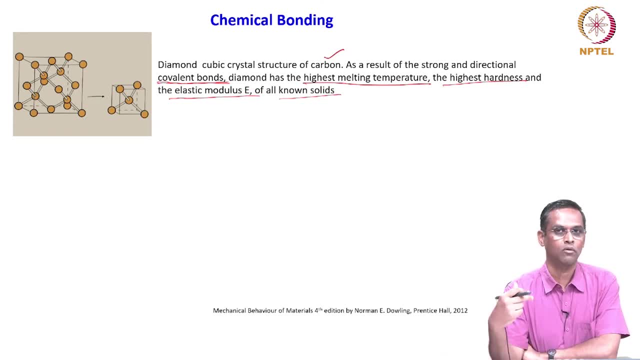 not necessarily only one. For example, even in water you had covalent bond between hydrogen and oxygen, but that is not uniform everywhere, it is just one bond. So that type of bond is also called hydrogen bonding. we will come to that, we will talk about it. 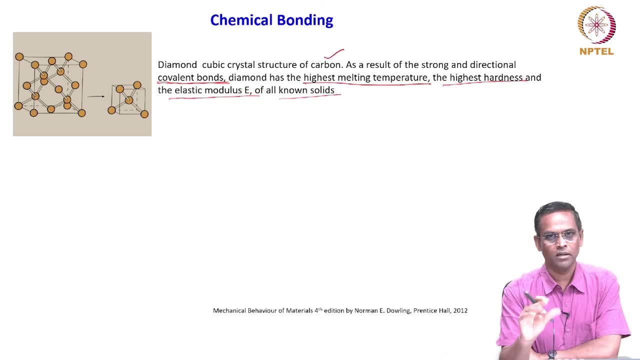 Do not confuse with that. So water has got a very. you can talk about dipole bonds, you can talk about hydrogen bond, you can talk about covalent bond. So water is very interesting solvent or interesting liquid. But what we here, we are talking about if you have a. 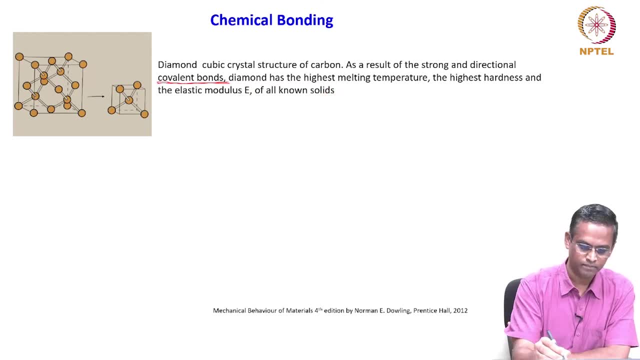 bond, uniform covalent bond with its neighbor. suppose, for example, if you take the single unit here, the each carbon has got you know, the tetragonal unit. So they are, all you know, covalent bond. So that is why they are very strong and a material which exhibit this kind of 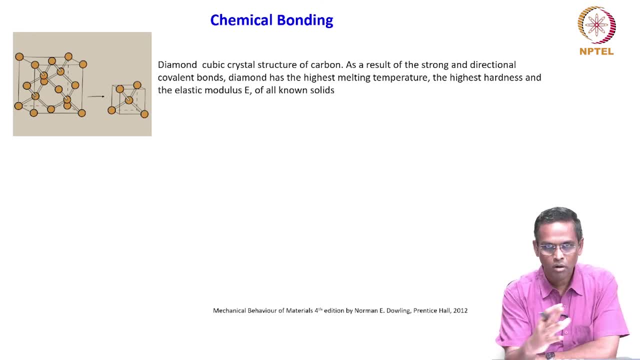 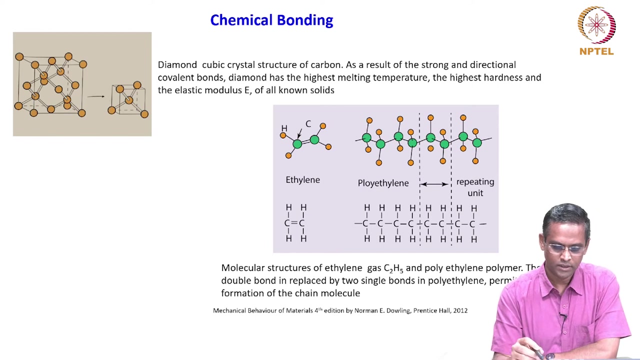 a directional covalent bond, uniform with its neighbor, which generally exhibit high melting point, high hardness and high elastic modulus. very important, right, elastic modulus. Okay then, coming to this, polymeric materials, which is what we are showing here, is ethylene and polymers are all molecular structures, right? 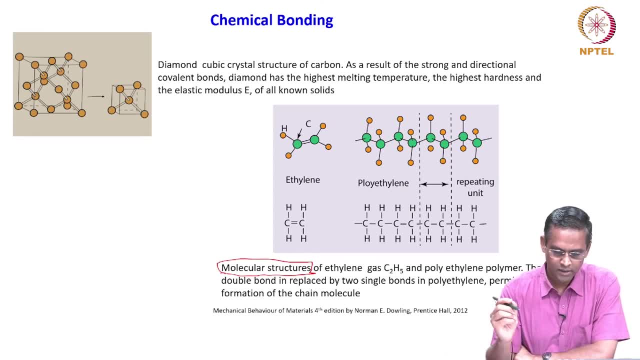 they are all molecular structures. Okay, this is a molecular structure of ethylene gas: C2H5 polyethylene polymer. The double bond is repeated by two single bonds in polyethylene, permitting formation of a chain molecule. So these are the two molecules. You see, so far we have just looked at atoms. 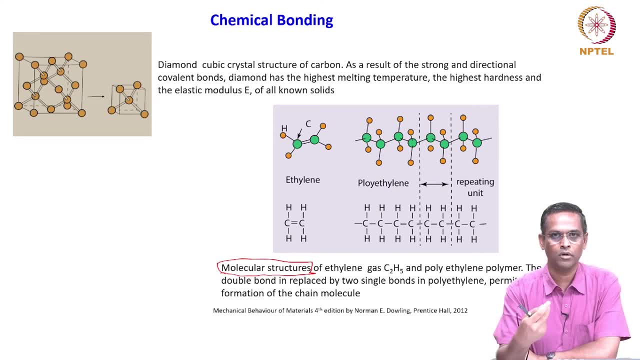 whether you talk about metallic bond or whether you talk about ionic bond, covalent bond. We were just talking the bond between atoms, but now here we are, switching over to molecular structures. right, So there is a difference. So, molecular structures. 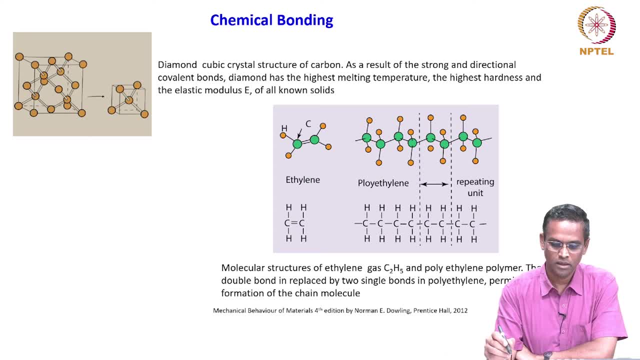 have chains, So mostly have chain molecules. Right, Polymers are all made up of chain molecules, So within this chain you have this carbon hydrogen, this covalent bond, and how these chain molecules are getting together or held together, that is again an interesting point of view you have to think. 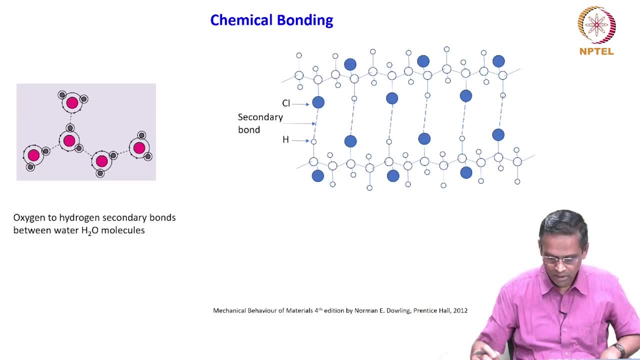 about it. So that is where we are going to discuss about this: secondary bonds. So the first one, what you are seeing here is again oxygen to hydrogen, secondary bonds between water molecules, So each one is water. So you see that hydrogen, this is an oxygen. 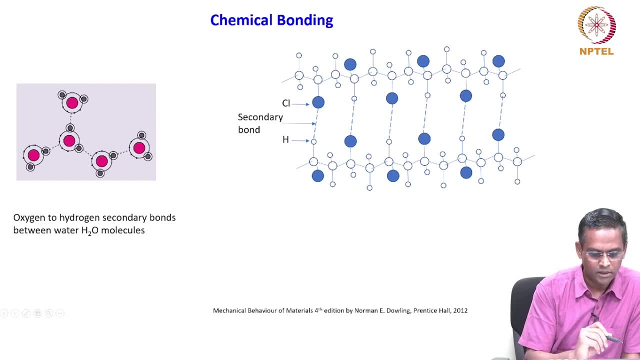 so there is a bond. These are all called hydrogen bonds. So these are the hydrogen bonds. They are vertical bonds. by vertical bonding, Like I mentioned, you can also have water also exhibits dipole, and here we are now not talking about that. there are any molecule which exhibits a dipole will also show a permanent dipole bonds. 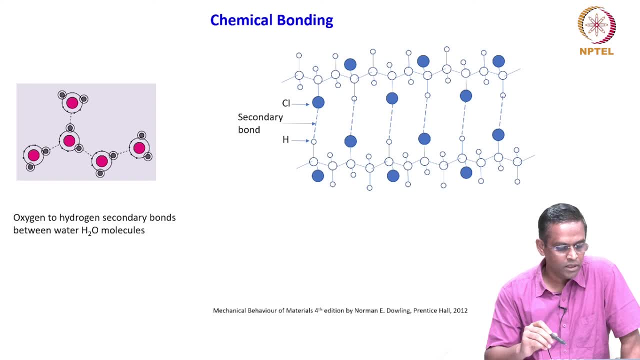 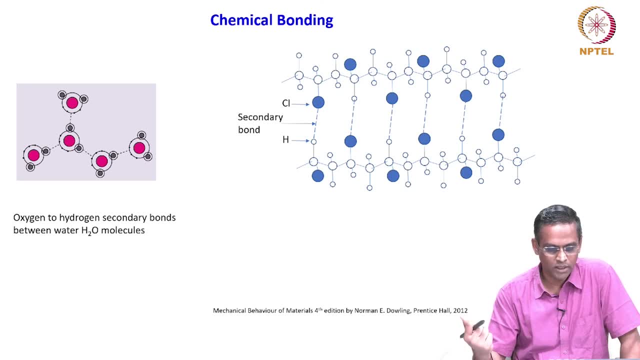 and you also have hydrogen bonds and dipole bonds, So most we are now here referring to hydrogen bonding. Similarly, if you look at this, hydrogen to chlorine, secondary bonds between the chain molecules in polyvinyl chloride. So this is one unit, this whole unit. 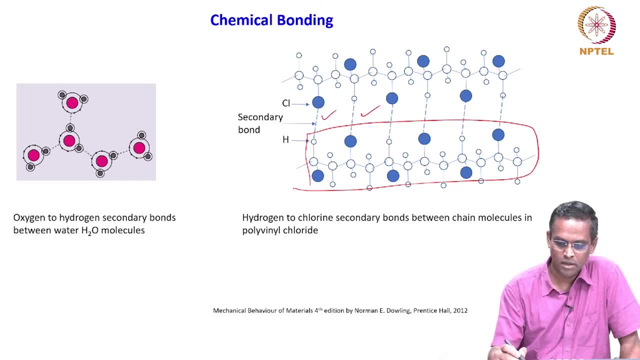 and this is another unit. they are all just held by this secondary bond. So this is hydrogen and chlorine, this is there are held between these two. So this particular schematic shows that you know, all the polymeric material are having primarily chain molecules and they are held together by Van der Waals forces or secondary bonds. 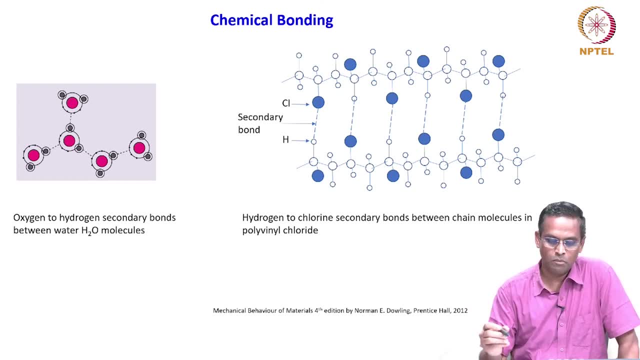 So that is how you should keep in mind. But the bonding between each of this carbon atom and hydrogen, they are all covalent bonds. So we will come when we discuss the you know the external force on each one of them, Then we will understand why this bonding is important, right? So, for example, the question 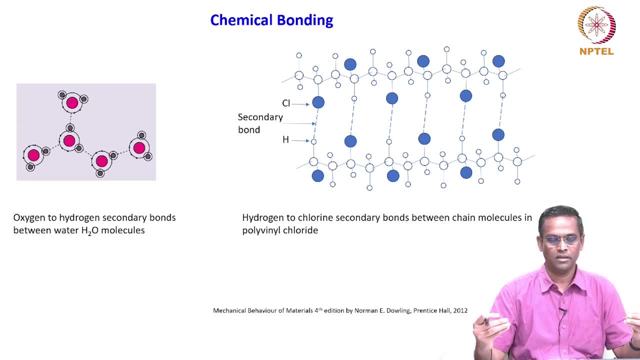 here is suppose, if I am just taking a polymeric material and then I am trying to apply external load, which bond will respond first right, which or which bond will resist to keep the material intact? or which of the forces will act against the external forces? That is the. 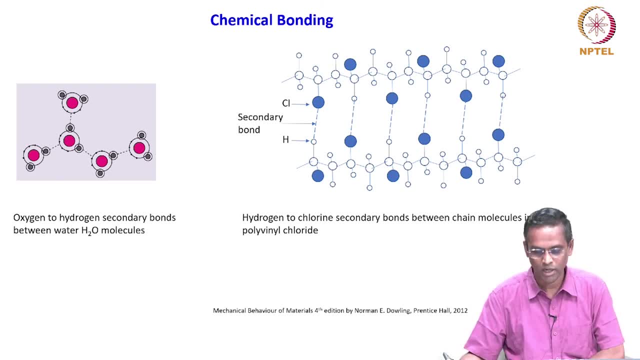 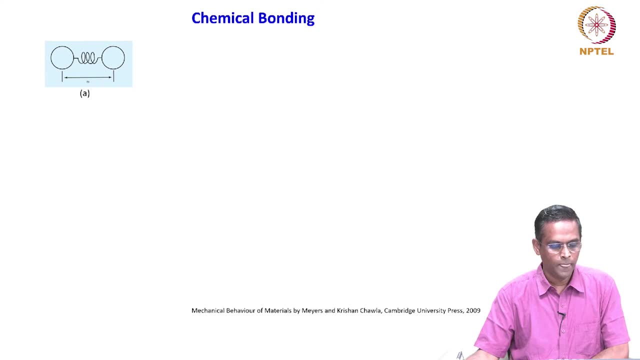 question right. So these are the aspects. we will look at it as we move along. So here is a model. consider two atoms. they are all held by some imaginary springs. The distance between these two atoms is r naught. That means the distance between these two atoms is r naught. That means the distance. 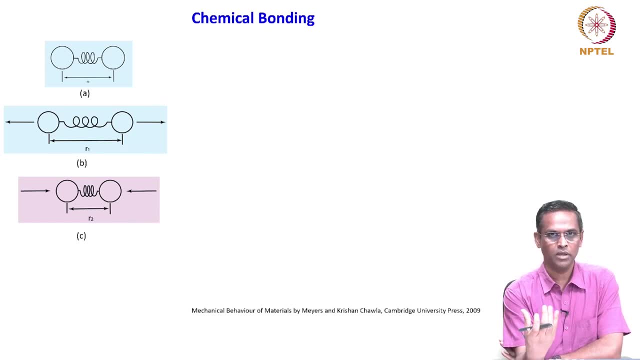 the two atoms are held together in an equilibrium position or stable position. And then the next image shows that these two atoms are pulled apart in a tension, so the R naught become R1, and the image C shows the two atoms are getting compressed the distance. 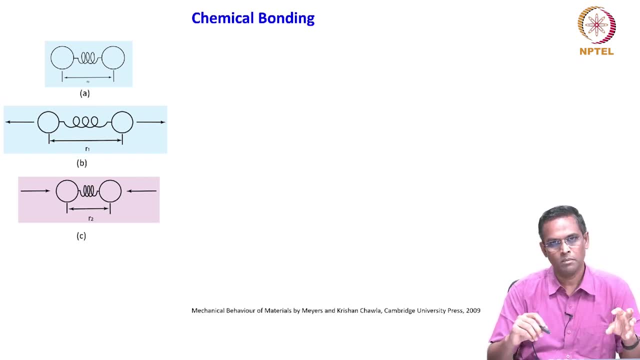 becomes R2.. Please remember all this deformation are within elastic units. right, we are talking about elastic deformation, So you are able to pull it in tension, You are able to compress the two atoms together. So what happens when you have these kind of two atoms which are held in equilibrium position? 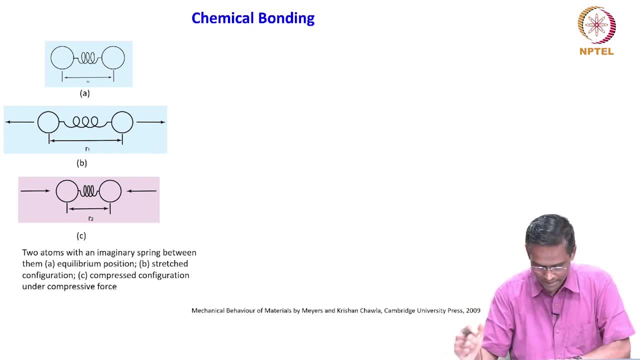 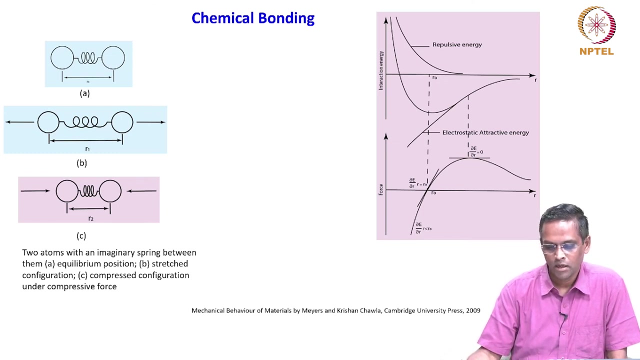 you try to pull it and try to compress it, what happens? So you can clearly see that there is something happens to the interatomic forces or interatomic energy, Which is plotted against the as a function of R. okay, So if you look at the top image and let us describe this, this is a plot between interaction. 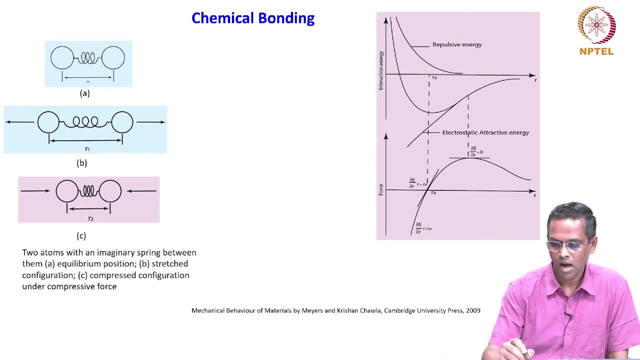 energy versus separation R. The top curve is repulsive energy, the bottom is electrostatic attraction. This is attractive energy, So the net force is in between. it is a potential bell or the potential bell- sorry, potential bell curve, that is. that is how it has been popularly known. 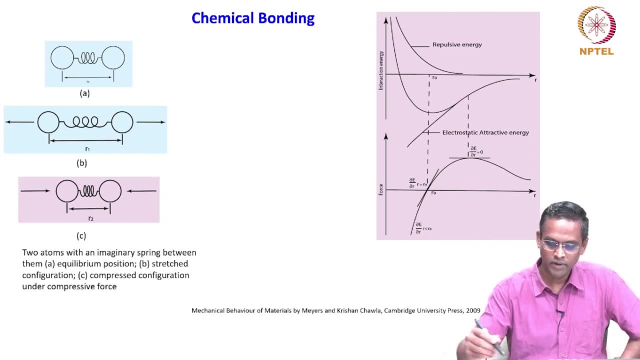 So when it is repulsive, when it is attractive, So when the as the separation goes up, Then the attractive forces are increasing, When the atoms are coming closer and closer and then the repulsion energy goes up. So it can be and you can also calculate the force. that is what shown in the bottom figure. 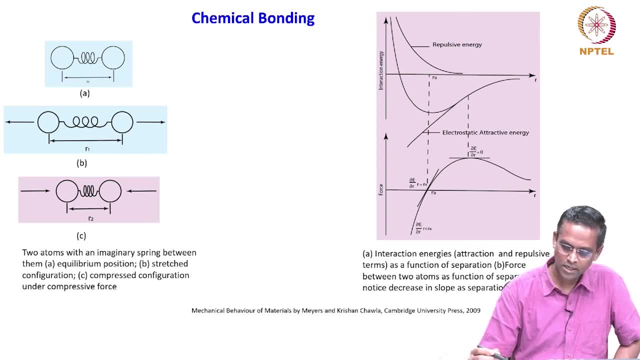 The force versus separation, The interesting point to notice. Okay, So if you look at this, the force is zero at R naught. there is no net. force is zero at R naught. That means when they add two atoms are in the equilibrium position. there is no force. 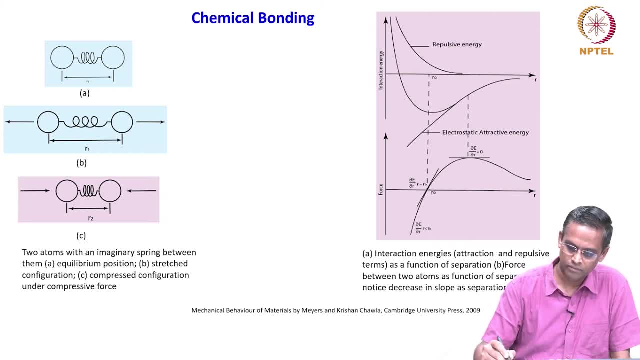 Okay, Then the as the separation between two atoms larger, becoming larger, then the slope changes and it reaches a maximum. So derivative is zero, Right? So? So the decrease in slope as separation increases, or slope becomes almost decreases and becomes zero. So the energy can be represented by the formula Ui: is equal to minus a, by R to the power m. 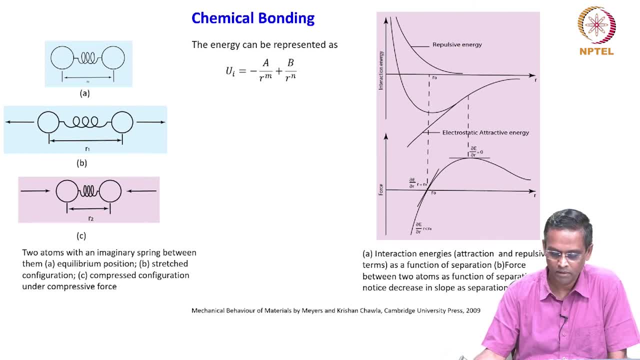 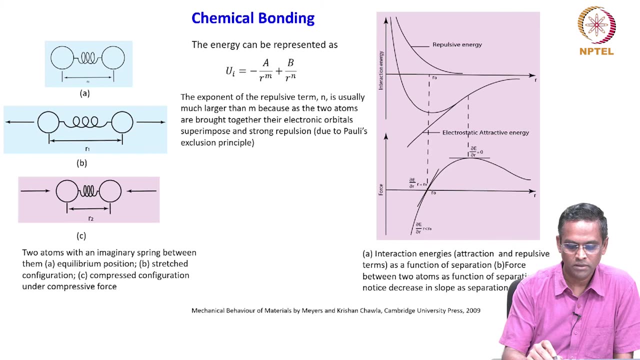 plus b by R to the power n. Okay, So the first one is Okay. Okay, So first one is attraction And second one is repulsion. Okay, The exponent of the repulsive term n this. this term is usually much larger than the. 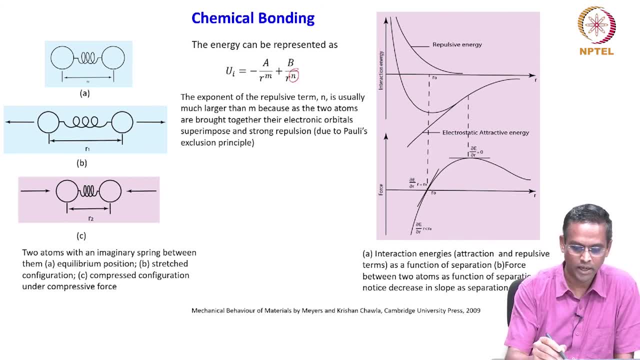 m. So because, as the two atoms are brought together, their electronic orbitals superimpose and strong repulsion as you go in this direction, this direction, direction, this curve, due to Pauli's exclusion principle. So this all we know, but we are now. 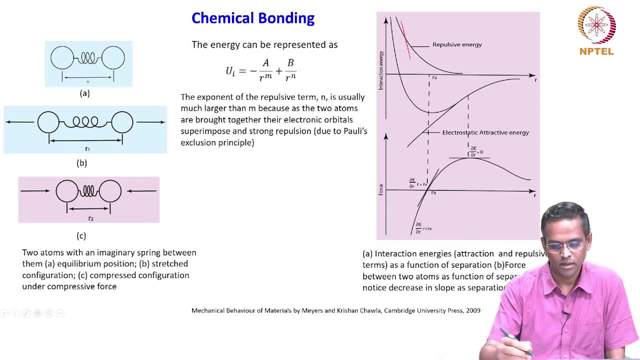 trying to connect all of them. So the inter atomic force is obtained by F is equal to dou Ui by dou R and, as is shown in this figure, the force is 0 at the bottom of the interaction energy curve. So here, if you look at this curve, it is a bottom we are referring to, that is, 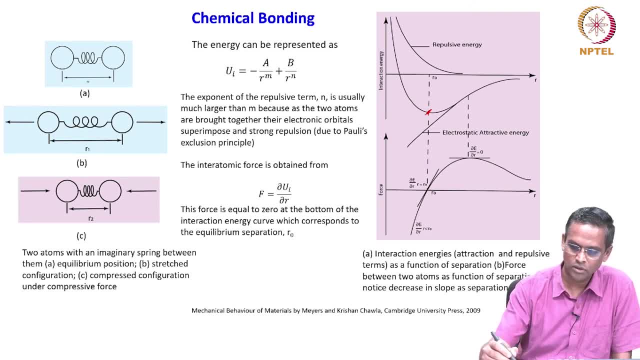 that is, the force is 0 at the bottom and which also corresponds to R naught here. So this we will. we are just introducing this curve here, but we will spend more time on this curve. it is called the Candon-Morse curve, So we will also connect this property. 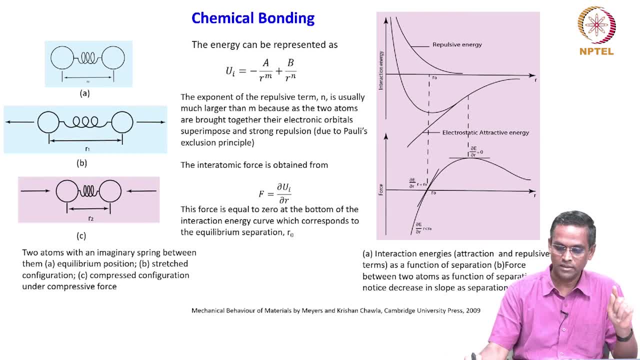 to the elastic modulus and we will also connect this to. you know atomistic, you know, I would say atomistic relation with its elastic properties. you know what is the atomic basis for the elastic properties of materials. So we will spend more time on this curve. 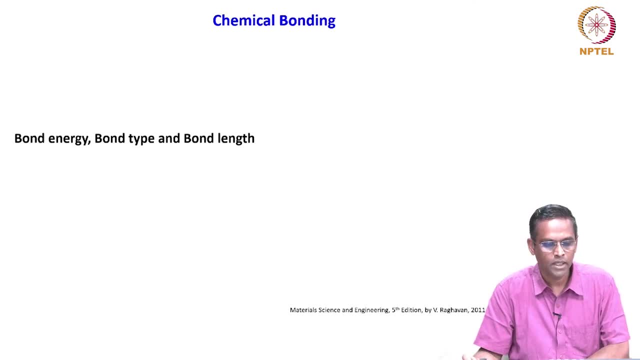 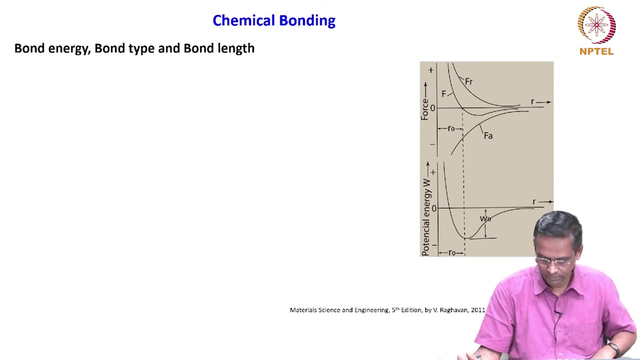 So this is just an introduction. So if you look at chemical bonding much more closely, So same curve here. this is F. R is a subscript, R is supposed to be subscript, A is supposed to be subscript. force, attraction force, repulsive force, right, So this is a equilibrium distance R naught. 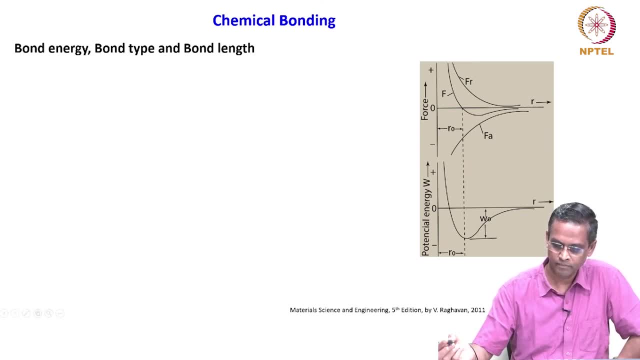 and this is a resultant force and this bottom one is a potential energy. the previous one, what we have just looked at before, is force versus separation, intra atomic energy versus separation. There are so many ways to look at the physical event right, so many ways. So here force is the. 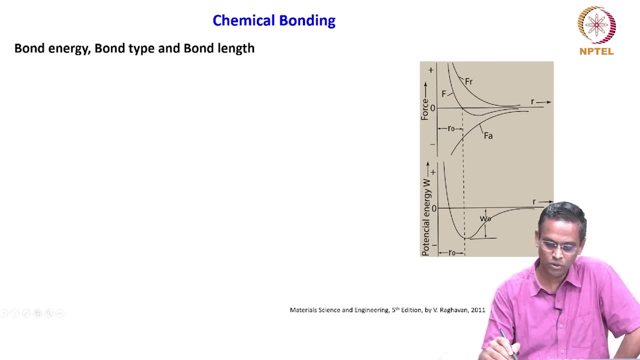 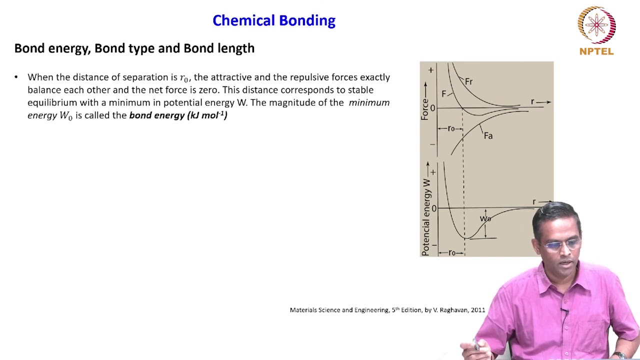 same force versus separation is there, but it is potential energy W versus separation. So we will try to look at bond energy, bond type and bond length. When do you say bond length? what kind of each bond has got a characteristic bond length, or each molecule is characterized with bond length? 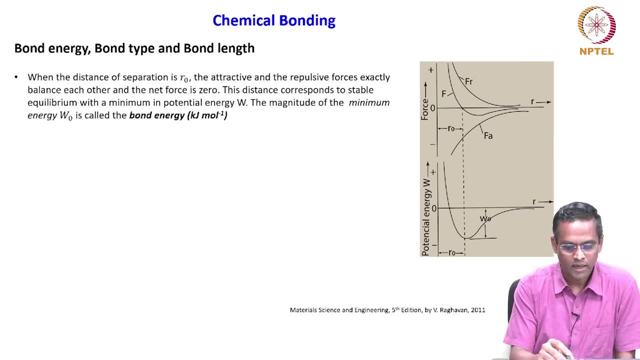 So when the distance of separation is R naught, the attractive and repulsive forces exactly balance each other and the net force is 0. this is what we have seen. The distance corresponds to stable equilibrium with the minimum in potential energy. the magnitude of the minimum energy, W naught, is called bond. 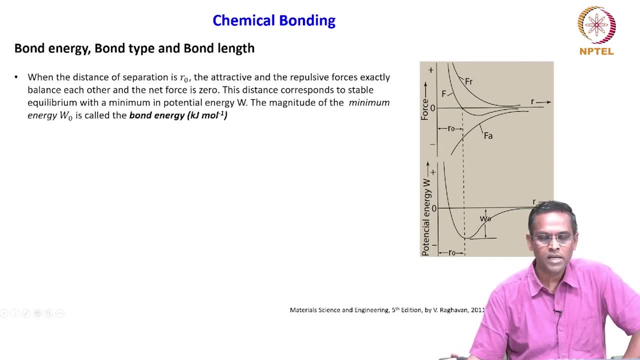 energy. So so we are bringing this potential energy versus separation curve to bring the idea of bond energy right. So what is that energy? That is the energy, the minimum energy, where the distance between the bottom of the potential well and the 0. So that is W naught is a. 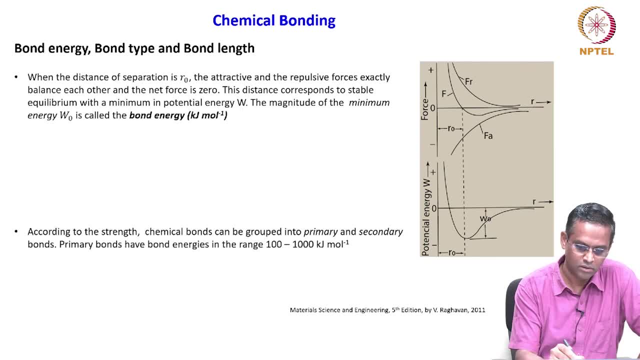 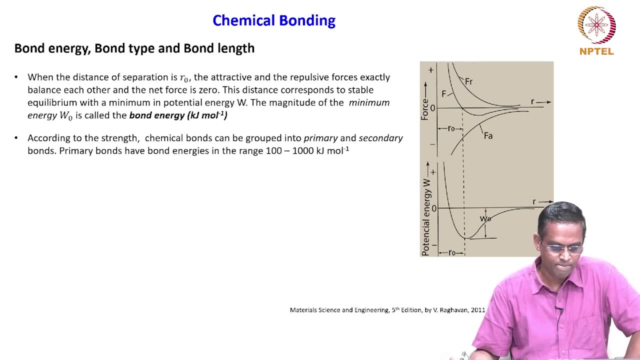 bond energy, which is measured kilo. the units is kilo joule per mole. okay, So according to the strength, chemical bonds can be grouped into primary and secondary. See this. we have already seen primary bond and secondary bond. And how about their energies? 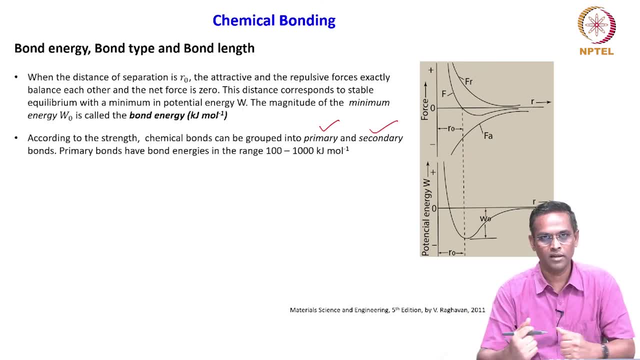 So that is the question Now we are going, because we are going to talk about mechanical response, right? So we start from this basic. The primary bonds have bond energies in the range of 100 to 1000 kilo joules per mole. 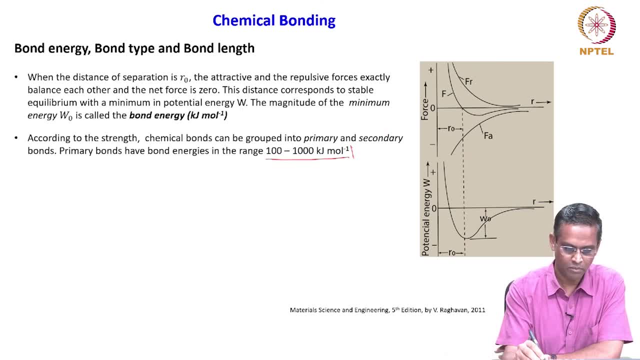 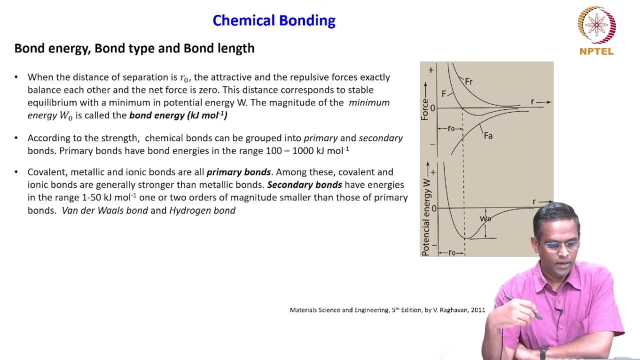 So this is a primary bond. So what are the primary bonds? They are ionic covalent metallic, So they are in the range of 100 to 1000 kilo joule per mole. okay, And among these primary 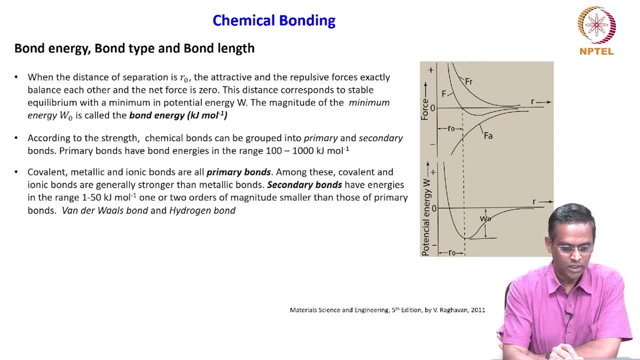 bonds. the covalent and ionic bonds are generally stronger than the metallic bonds. So very important, So very important. So we have to keep that in mind. Covalent and ionic bonds are stronger than the metallic bonds. okay, 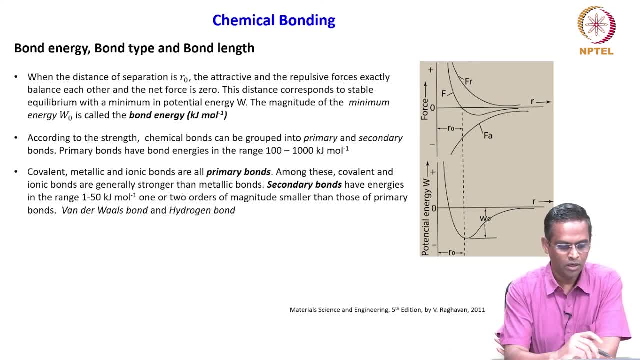 Secondary bonds have the energies in the range of 1 to 50 kilo joules per mole. okay, It is much lower than the primary bond, energies One or two orders of magnitude smaller than those of primary bonds. And the examples we have already seen: van der Waals bond and hydrogen bonds. they come. 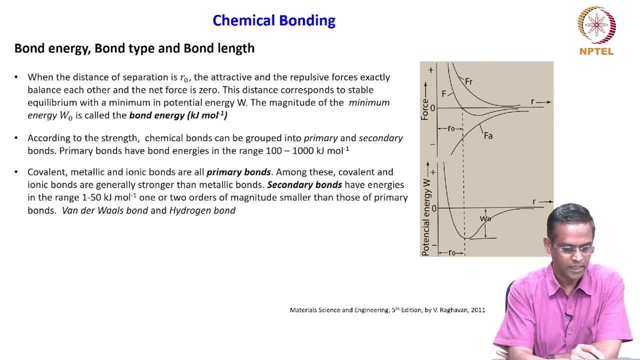 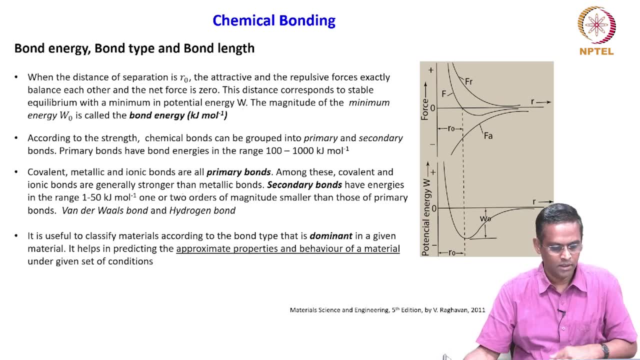 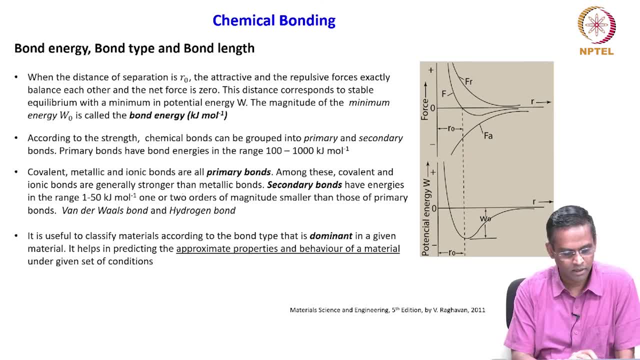 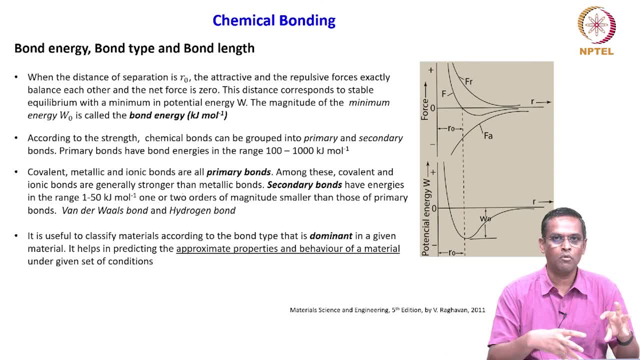 character. that is what it means. one can have, you know, ionic bond and metallic bond, ionic and covalent. So which will dominate, suppose, if I have a material which has the characteristic of ionic and covalent, or ionic and metallic, So which character is dominant? So that is what. 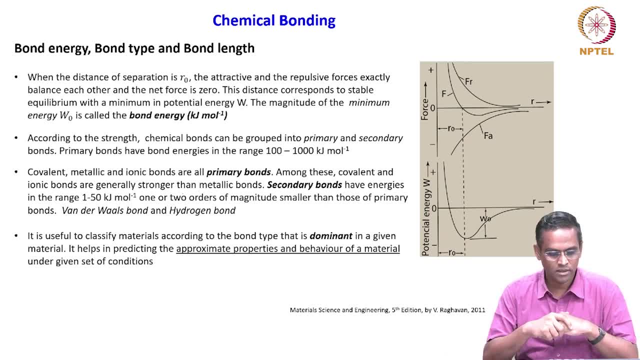 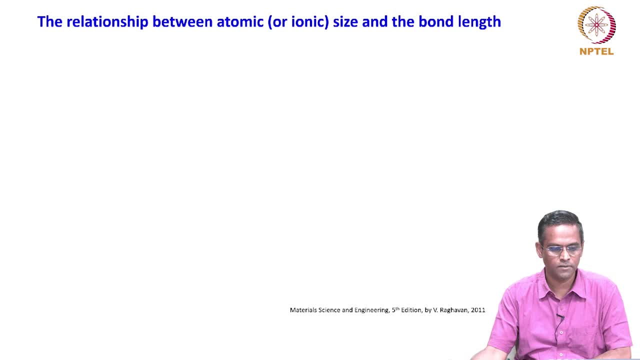 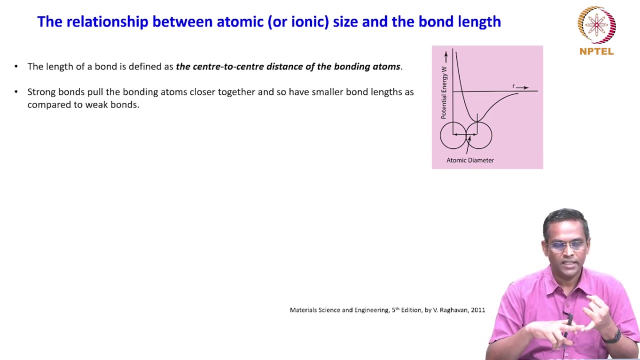 means here. So if you know that, what is the type of dominant bond, then it will again easier to predict the behavior under the set of conditions. So the relationship between atomic size and the bond length. So we look at bond energy and bond length. and types, bond type. So now we look at bond length and atomic 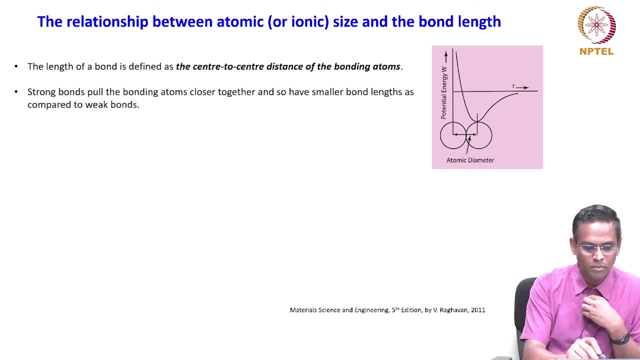 size how they are related. The length of a bond is defined as the center to center distance of the bonding atom. So again, we will refer to this potential. well, curve potential energy versus R. So when the the distance between the two atoms is R, naught the center to center distance is bond. 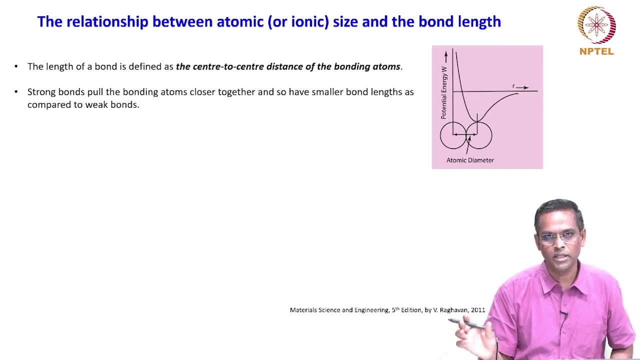 length. So that is when atoms are at equilibrium position or not. then the center to center distance is called bond length. So strong bonds pull the bonding atoms closer together And so have smaller bond lengths as compared to the distance between the two atoms. OK, So when you have an atom and 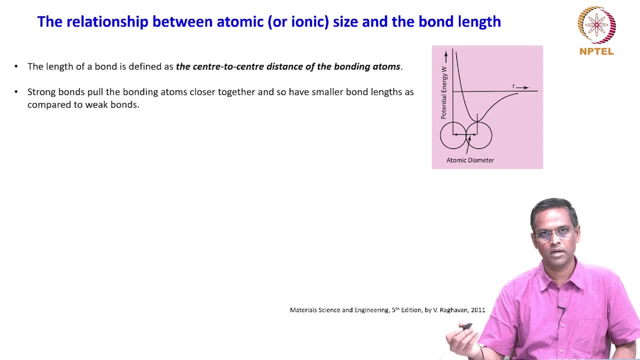 the resistance between the two atoms is called bond length. So when the distance between the two atoms compared to weaker bonds, So this is quite understandable, right? So we have now seen the bond energies, right So, how strong they are, So they will try to hold together more. 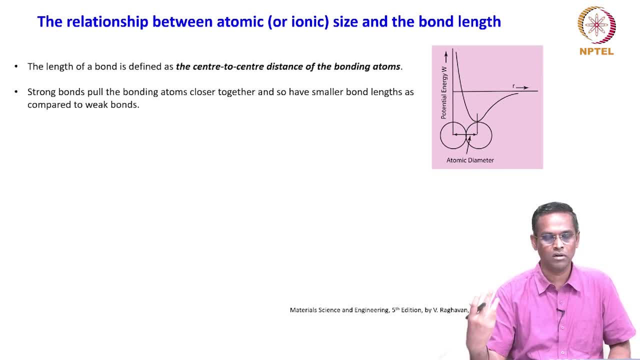 tightly than the weaker bonds like van der Waals or hydrogen or dipole bonds, right. So for primary bonds, they have the lengths in the range of 1 to 2 angstrom or 0.1 to 0.2 nanometers. Secondary bond lengths: they are much larger, in the range of 2 to 5 angstrom. 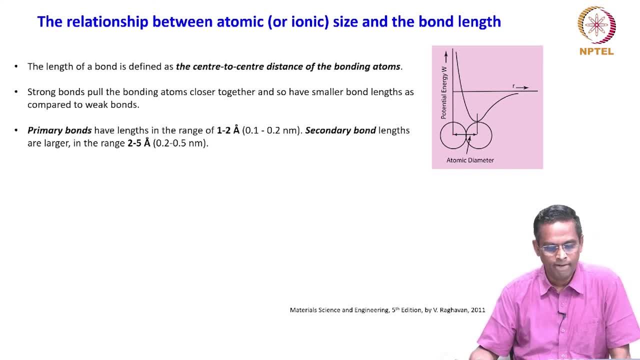 or 0.2 to 0.5 nanometers. So very important to keep this. So this is a very important point, So this is a very important point, So this is a very important point, So this is a very interesting point, When the bonding is between two neighboring atoms of same kind, the atomic. 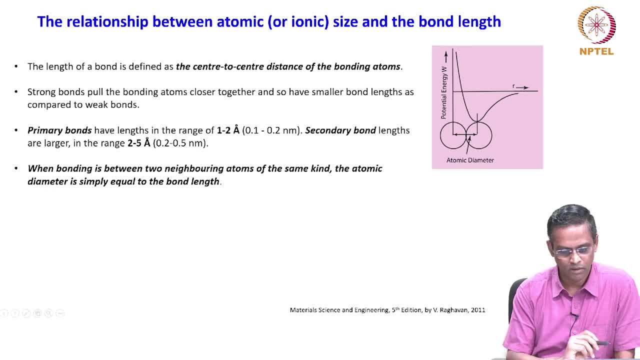 diameter is simply equal to the bond length. okay, So suppose if you do not have a similar atoms- right, you can have a solid solutions, right? or you can have ionic solid like sodium chloride and so on. where you do not have same type of atoms, you have different types. 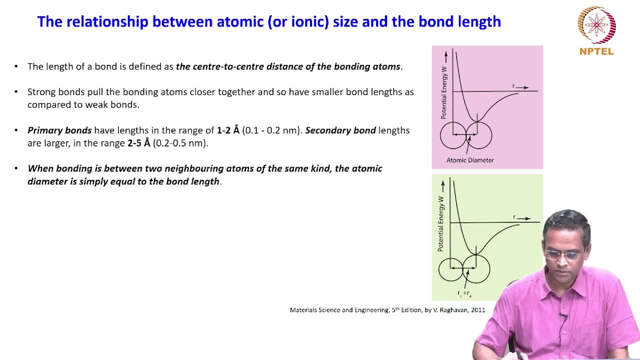 of atoms together, Then what happens? Then you look at this similar potential energy versus separation curve for atoms of different kind. One is, you know, for example, ionic solid. So this is anion and this is a cation. So Rc plus Ra, This is radius of cation and plus radius of anion. 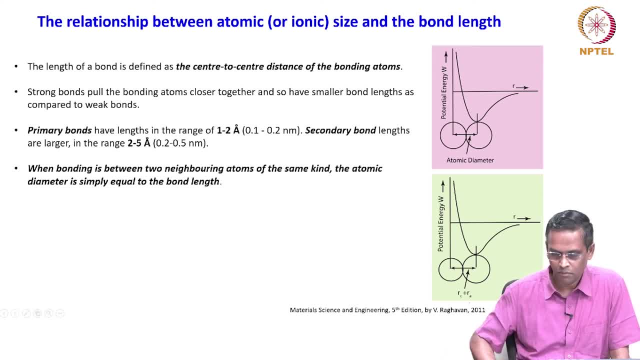 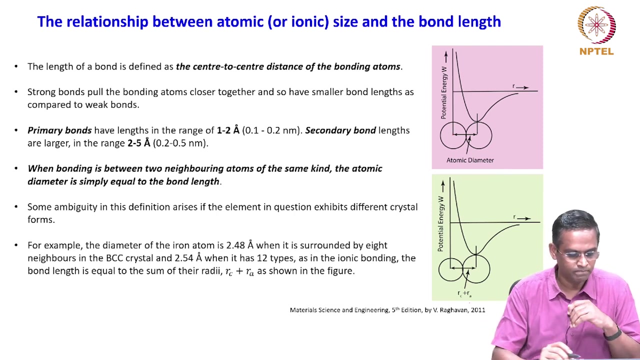 So this distance is the bond length. So that is why there is some ambiguity in this definition arises if the element in question exhibits different crystal forms. So another question: it is not necessarily anion cation issue If it is same material exhibits a different crystal form, for example the diameter of.